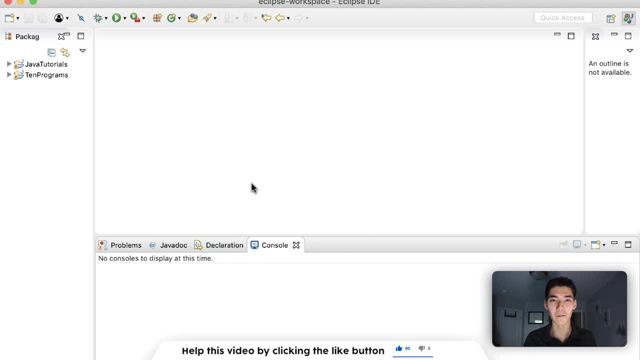 classes were pretty confusing. I'm pretty sure I didn't know what abstract meant when I learned them. My name is Alex. I make a Java tutorial on this channel every single week, so if you're new here and you might be interested in seeing that, then please consider subscribing. Let's start. 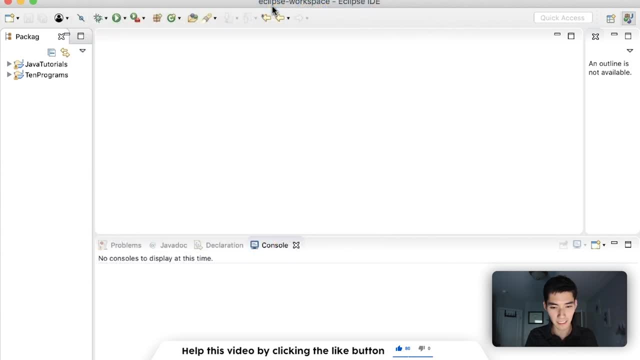 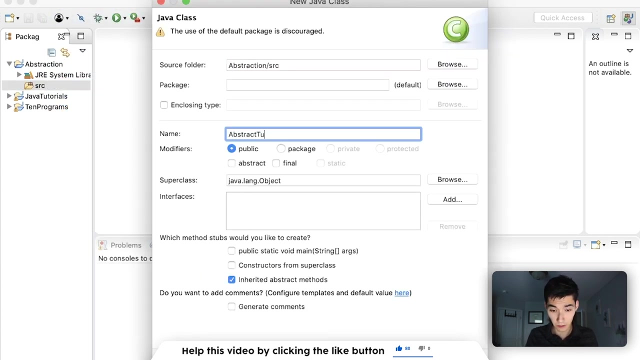 getting an abstract class here by going to file new java project, Call it something like abstraction, and then hit finish and on the source folder go into new class and we'll call it abstract tutorial. Hit this main method check box and then hit finish. An abstract class is. 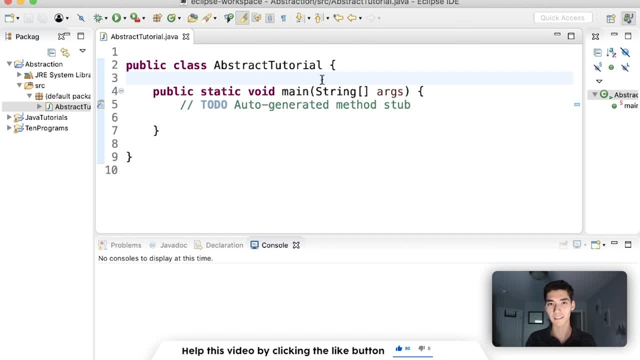 basically a bunch of variables and methods that can be used to create other classes. So here we can make an abstract class by doing abstract class. name is something like dog and what are some values for dog? well, we could have like breed or something. and what can a dog do? well, we could say bark, we'll have it be a normal method and 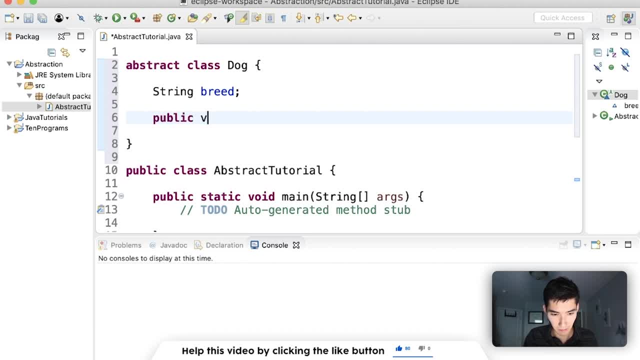 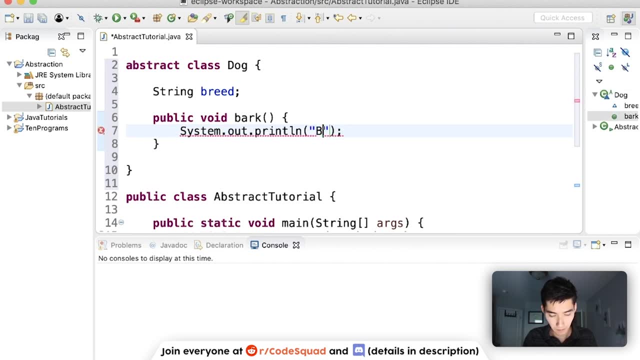 we'll actually implement it too, so we could say public void bark method. we'll print out bark like that so we can try to use this abstract class by doing dog d equals new dog and then trying to use it just like any other class: a dot bark. 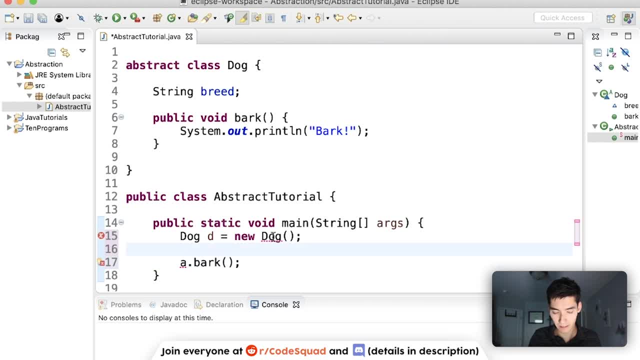 but it's looking like we've got some red underlines and let's see what the error is- cannot instantiate the type dog. if this was a regular class class dog, then you would see the underlines go away and we could do dbark and that would call it bark. 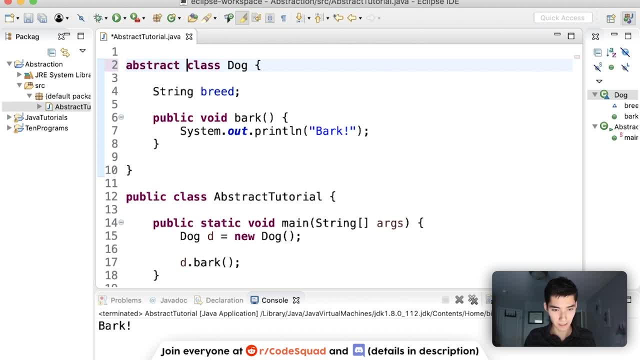 but as soon as we turn this into an abstract class, we cannot use it. that's because you can't use an abstract class like a regular class. an abstract class helps make regular classes that you use there, so we can create um a new class, class chihuahua. 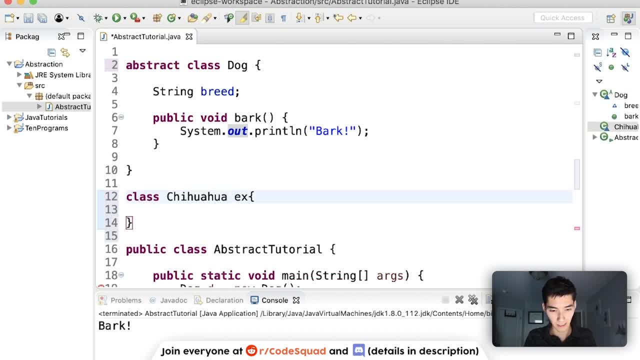 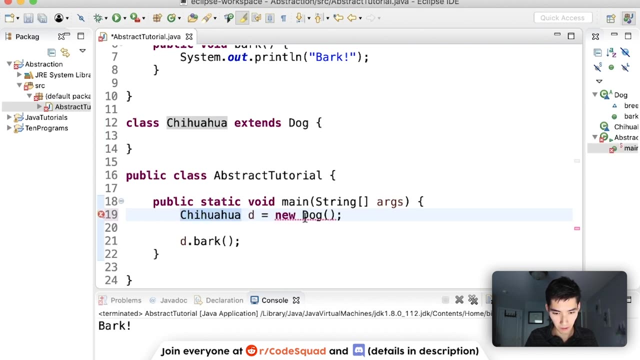 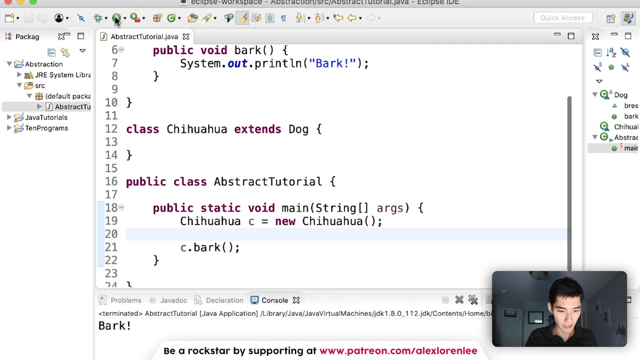 chihuahua class okay, and say: extends dog. so now we can use these through the chihuahua. so we could say: chihuahua d equals new chihuahua and i'll name it c for chihuahua. and now, if we do that, it'll work, because now the chihuahua object is an extension of dog. 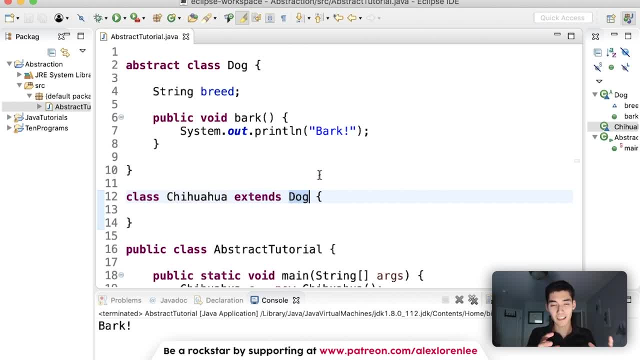 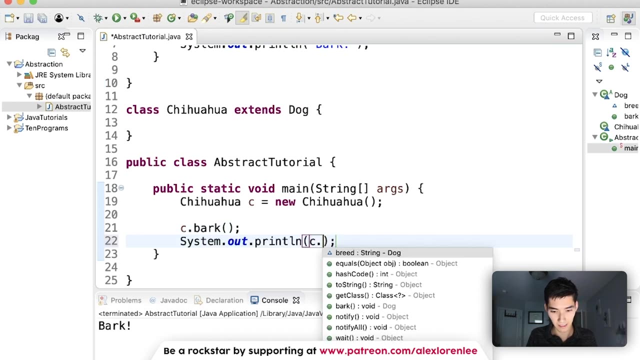 so if it's an extension, then it already has what the dog comes with and a little more. we just decided not to add anything, so the things it already comes with is a breed and a bark. so we could also print out c dot breed if we wanted to. this is known, because we're not setting it or using. 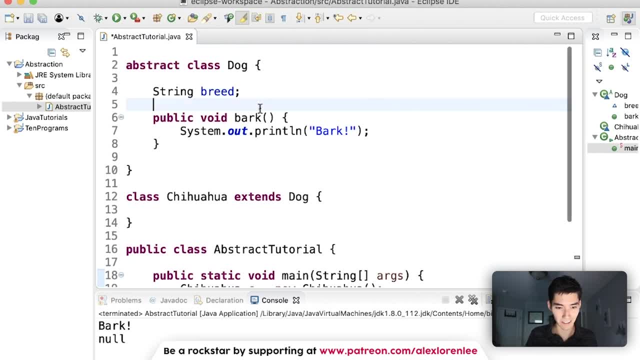 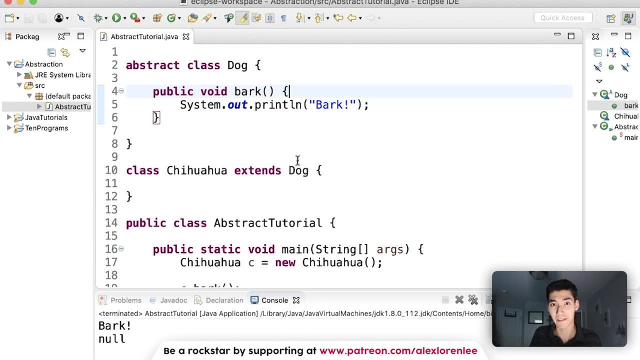 it yet, and let's actually get rid of that together, because this is the most important part of the important part about abstract classes in java: it's abstract methods. i'll close this up so we can see everything a little better. an abstract method is a method that isn't implemented yet. 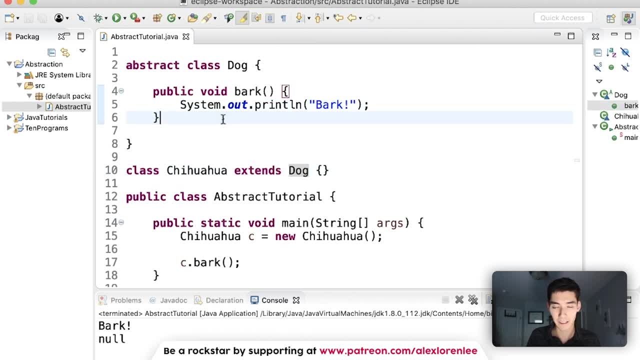 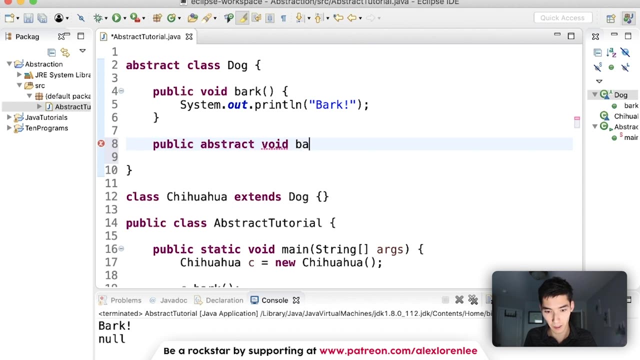 so implemented means you put code inside the curly braces. we're going to make an abstract method, which means we're not going to put code inside the curly braces. so it's the same as before- public, except we add this new keyword, abstract, public, abstract void bark. so we want to do it this way. actually, we'll change it to poop poop. 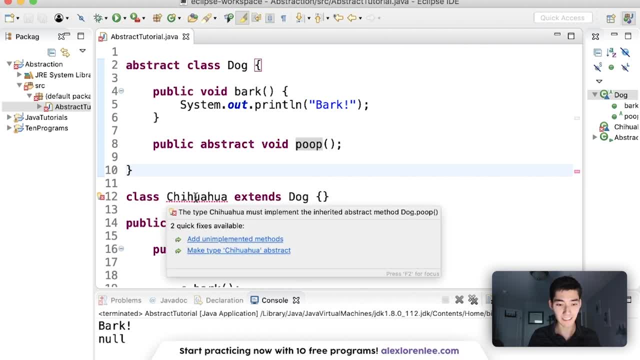 now we get a red underline under chihuahua because it needs to now have the poop method, since we're extending it. we don't have to add the bark because it's already implemented here. there's already code, it knows what to do, but now we have this abstract method which doesn't know. 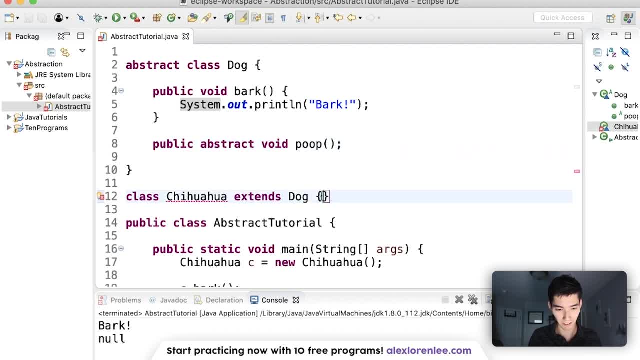 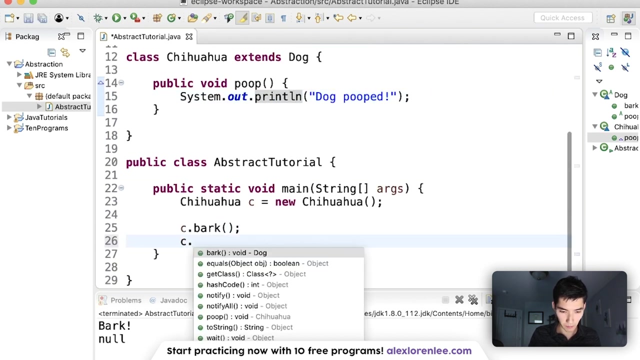 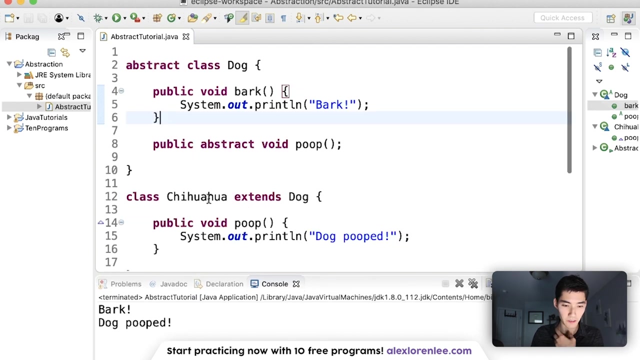 what to do when you call it. so we have to say what it does when you call it. so we can now say: public void poop. we want to print out dog pooped, okay. so now, if we do cbark and cpoop, then we'll see both of those messages. so chihuahua knows how to bark, because it extends dog. 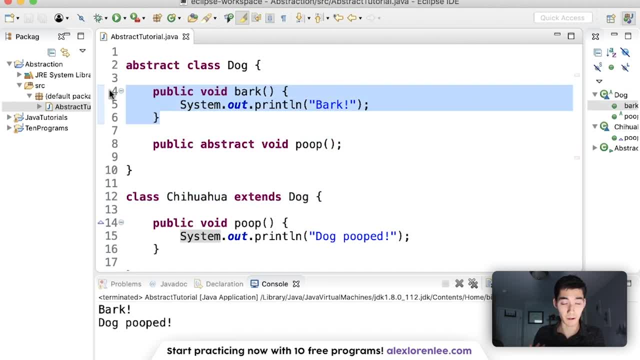 it knows everything inside of here, which is why we can call chihuahuabark. it also knows that it needs to poop, but it doesn't know what to do since it's not implemented. and that's what an abstract method is. it's abstract, it's an. 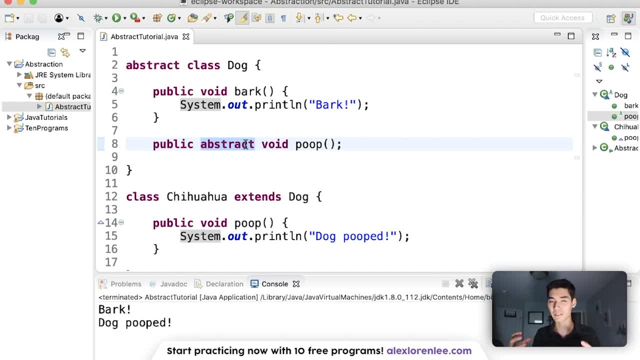 idea. it has to have the poop method, but it doesn't know what to do, so you need to implement it, which just means make the method poop and put code in it, and that's why it works. we could get rid of this abstract method and just add it like this. so if we ran it, it would say that's why it's abstract method. 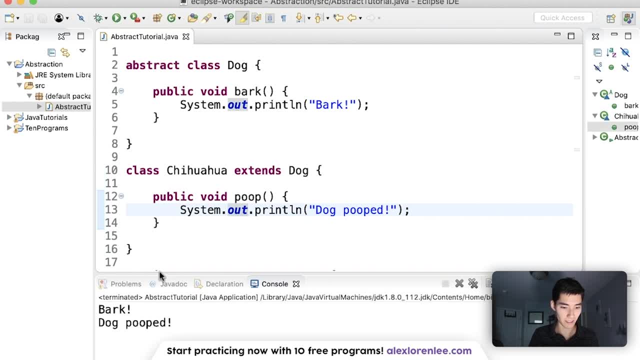 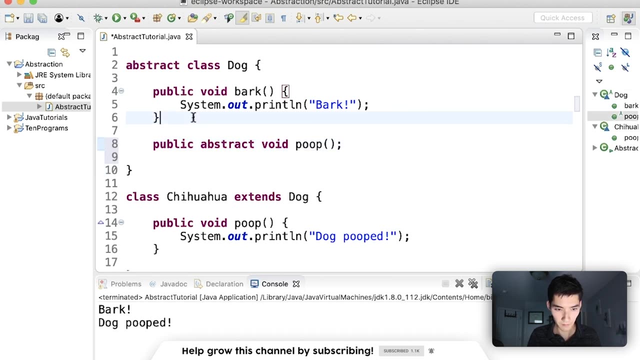 and just add it like this: so if we ran it it would still work. then you'd be like: well, why do we even have that abstract method in the first place here? well, abstract classes help us organize what a dog should have. what should this class be able to do? so we can just list out and make sure, make 100 sure that every single dog has. 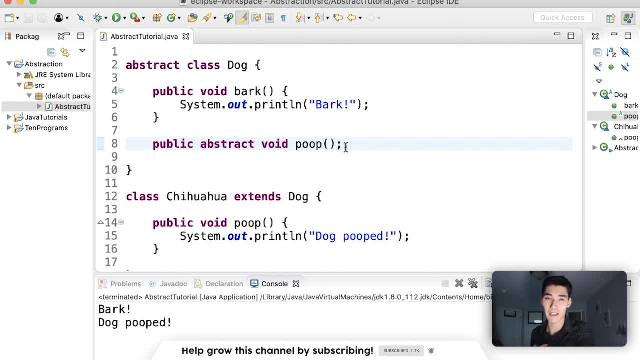 to have this method. it might be a very simple method. it would be a good method. if we have dog, It might be different for other dogs, so that's why we make it abstract, So each specific dog can poop a little differently or bark a little differently. 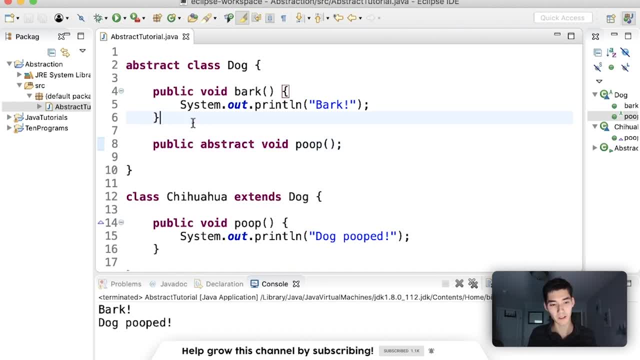 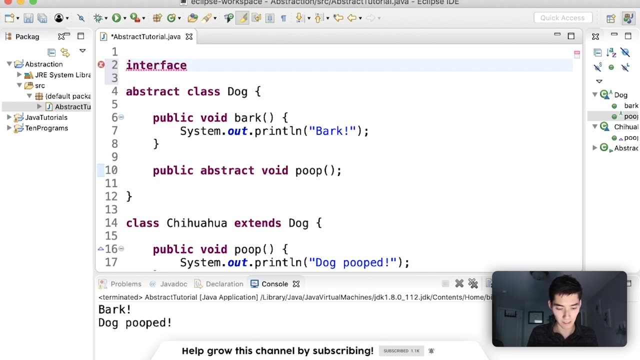 Basically, it's saying: you have to implement your own poop method, But all dogs, all these dogs will bark. the same is what this example is. So how is this different than an interface? An interface is like this: You type interface and say dog interface, for example. 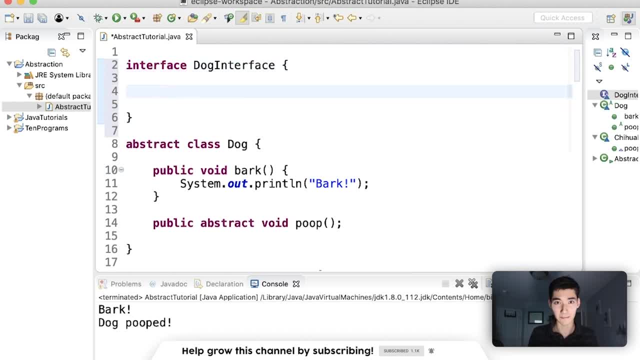 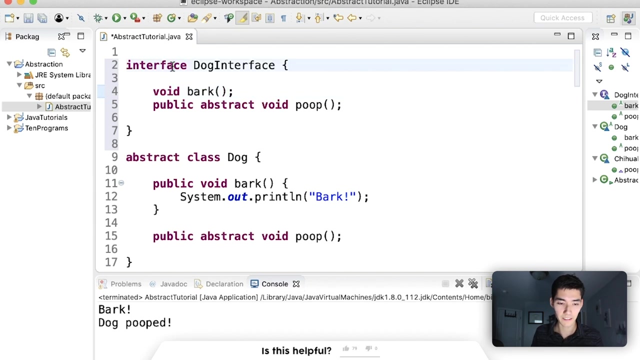 An interface is just a list of variables and methods too. So we could have bark and poop, void poop, But we don't have to put abstract here. We can, but an interface assumes that all of them will be abstract, which means unimplemented here. 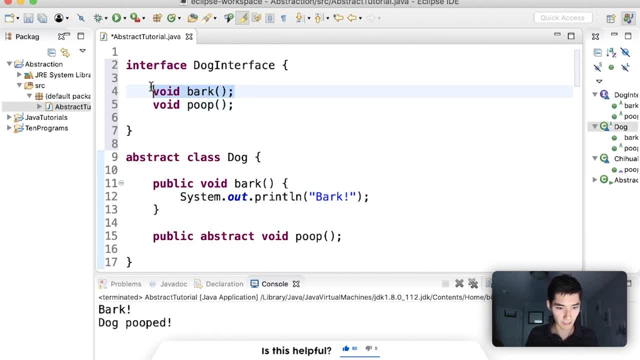 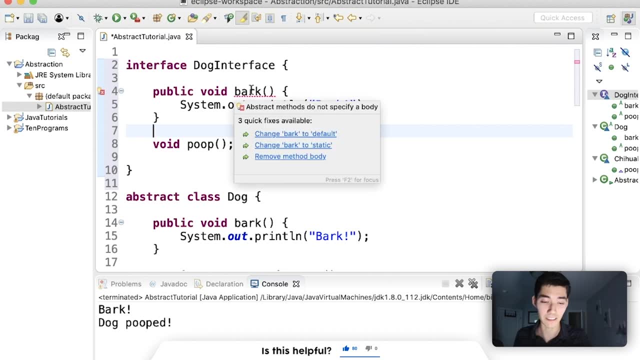 If we tried to implement an interface, to implement it here, just like in the abstract class. if we tried to do that inside of an interface, it wouldn't work. because look at the message here. It says: abstract methods do not specify a body.